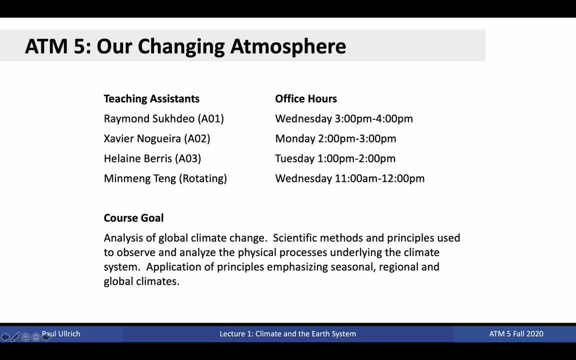 underlying the climate system and we're going to apply these principles to emphasize seasonal, regional and global climates. In order to contrast this against other climate change classes you may have taken or may be interested in, we're going to be focusing on the climate. 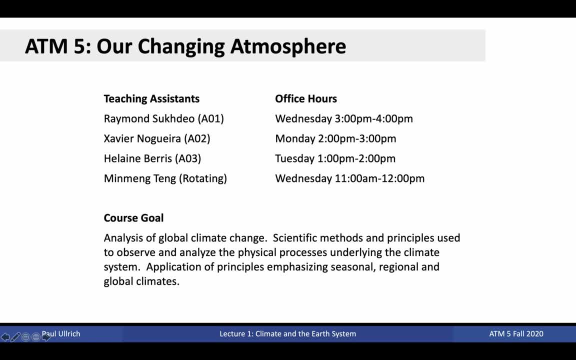 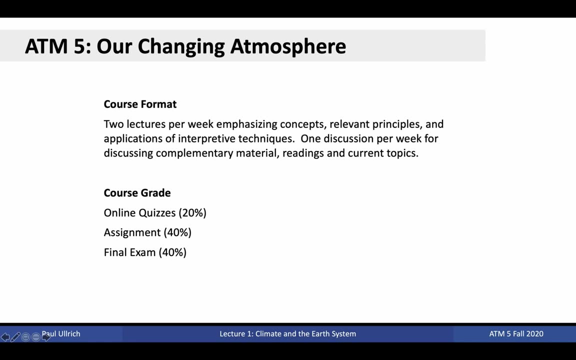 system. This class focuses heavily on the science of climate change. That is, we're going to focus on the physical system and understand how humans can influence that physical system and the consequences. The course format is two lectures per week. We're going to have both asynchronous. 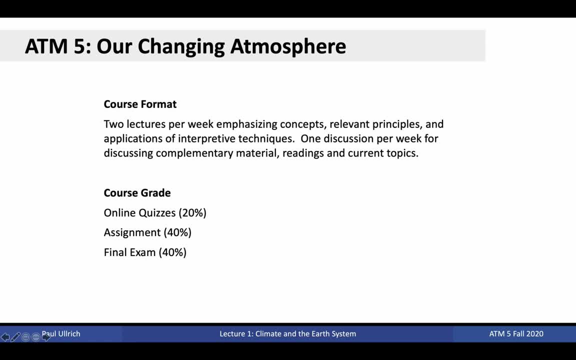 and synchronous lectures. Both the asynchronous and synchronous lectures will be covering the same topics and these lectures will emphasize concepts, relevant principles and applications of interpretation. We're going to be focusing on the science of climate change and we're going to be focusing on the science of climate change and we're going to be focusing on the science of. 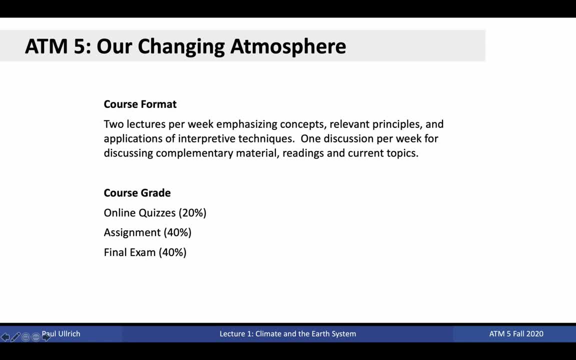 techniques. There's also one discussion per week, again depending on your section, for discussing complementary material readings and current topics related to climate change. The overall grade will be computed as 20% from online quizzes. There'll be one quiz associated with every lecture. 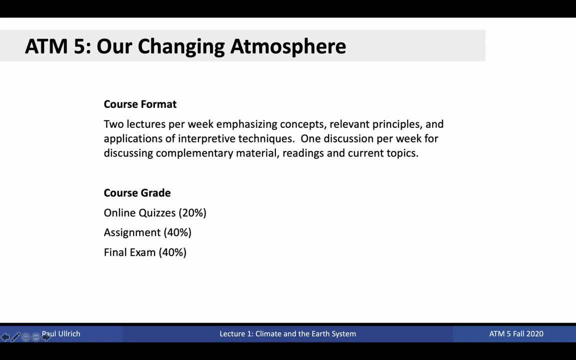 of the class: 40% assignments- There are going to be eight assignments total for the class and they'll be weighted equally- And a 40% take-home final exam, of which you'll have a few days in order to complete the final exam material and it will be cumulative. 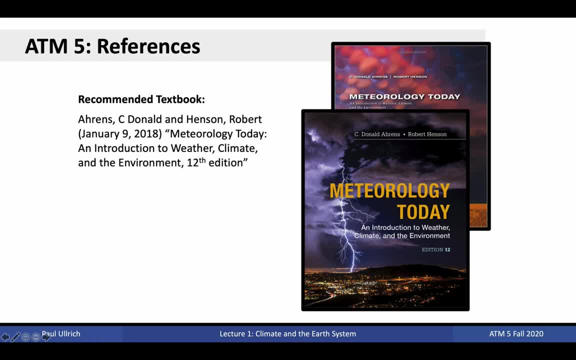 The recommended textbook for this class is Donald Aaron's book Meteorology Today, currently in its 12th edition. This book, I would say, is an excellent reference for understanding the Earth's system. Note that we do not follow this book particularly closely throughout this class Most. 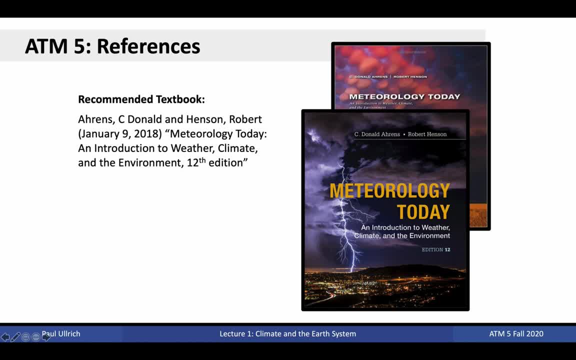 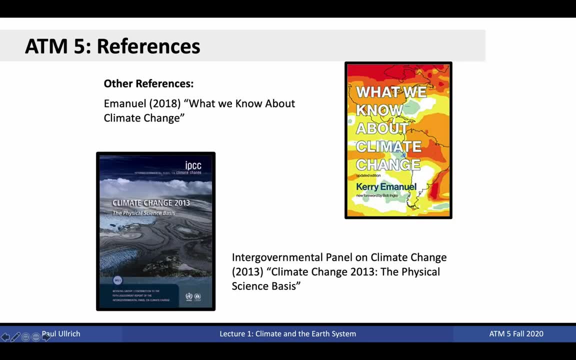 of the material is fairly customized for this class but nonetheless, if you are interested in having a second source for understanding the course material, then I'd recommend getting yourself a copy. Other references in case you're interested in learning more about the course material are the following: 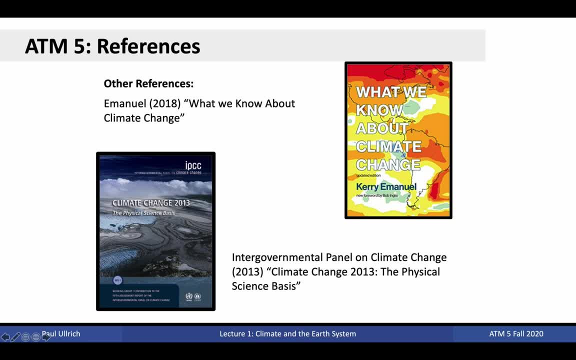 If you're interested in a pocket guidebook about climate change, I recommend Carrie Emanuel's book What We Know About Climate Change, with a new edition having been released recently in 2018.. This, I'd say, is a handy primer on the course content, and it could be read completely in only 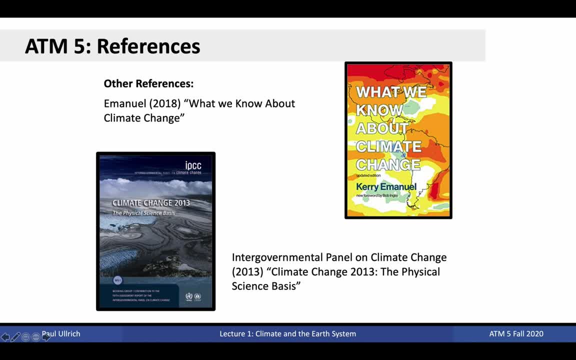 a couple hours. It's essentially just a pocketbook on everything we know related to climate change. It's a bit more than $10 on Amazon, so if you want to get spun up quickly on the course material, this is a good place to look. 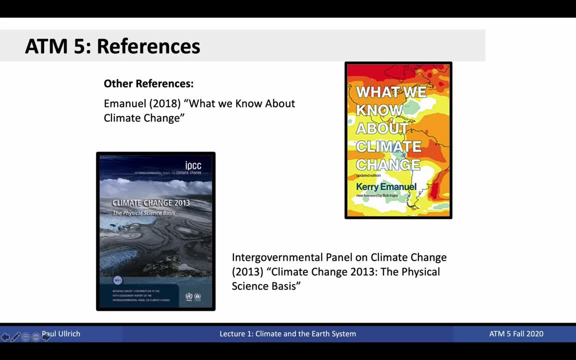 The science of climate change is all very well-understood, so as well. all of this we know has accumulated by our Intergovernmental Panel on Climate Change. Its Assessment reports, which are compiled every five to seven years, are a wealth of information related to climate. 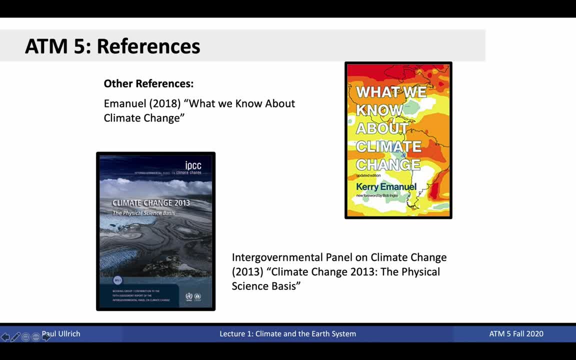 change. Some of that can be quite intense, I should say. So you can delve in and examine some of the easier material first before taking on some of the more challenging concepts. The Responding Propunkty by Mad évidemment Lohis 앞으로. 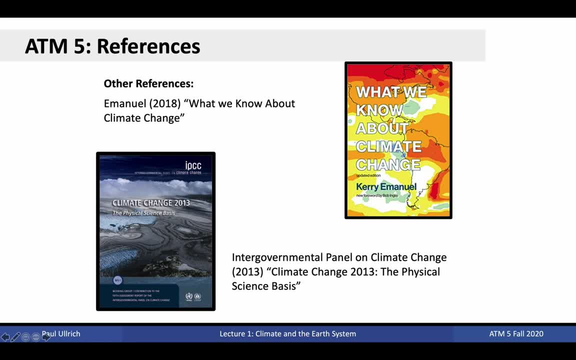 published report from the IPCC is the fifth assessment report, or colloquially called the AR5,, which was published between 2013 and 2014.. Now it is a little bit dated relative to 2020, but all of the science that from 2013 and 2014 still holds today. We've learned a little bit more. 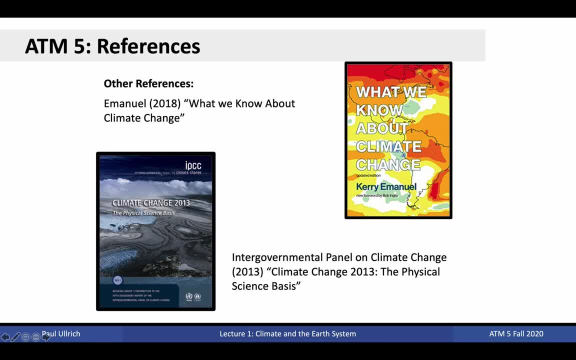 about climate change and some of the more nuanced aspects of how it's affecting the Earth system. but for everything you need to know in this class, the fifth assessment report provides you with what you need to know. The next assessment report, the AR6, was not out quite in time for this class. 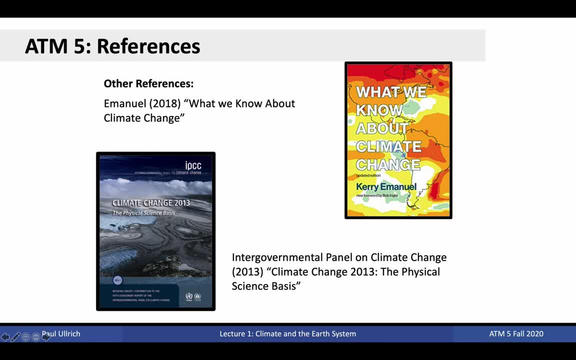 We anticipate it will be published in the beginning of 2021 through the beginning of 2022.. Nonetheless, the AR5 and earlier reports are going to be a handy reference for learning this material, and some of the readings that we'll have in this class will actually be drawn from these. 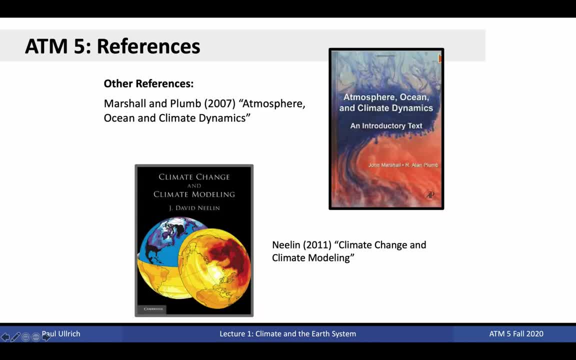 assessment reports. A couple more references for those interested. Marshall and Plum's 2007 book Atmosphere, Ocean and Climate Change is a great reference for learning about climate change. It is an excellent reference on how the Earth system operates and is actually the textbook for. 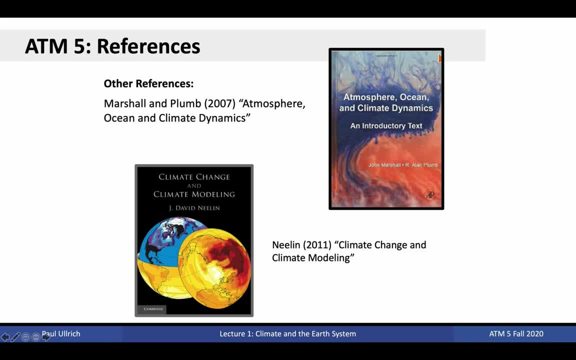 my graduate-level class on climate dynamics. If you aren't afraid of mathematics and want a deeper understanding of how energy and moisture move around the Earth, you can grab a copy of this text as well, And you can even follow along with my YouTube lectures on climate dynamics. 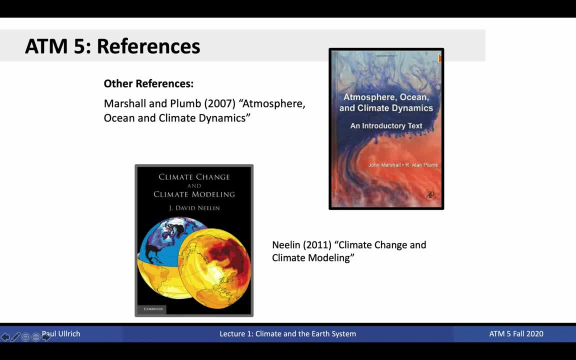 which are on my YouTube channel, which I'll bring up momentarily. Finally, in terms of physical reference books, we have David Nealon's 2011 book Climate Change and Climate Change. This is an excellent source of information on how we've used climate models to delve into the 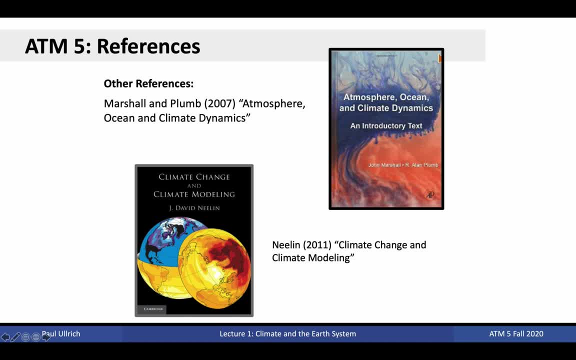 science of climate change. As a climate modeler myself, I'm, of course, a little bit biased towards understanding and employing climate models, and so I may bring them up here and there throughout the course. This book, however, I would say, is a great reference, in case you're. 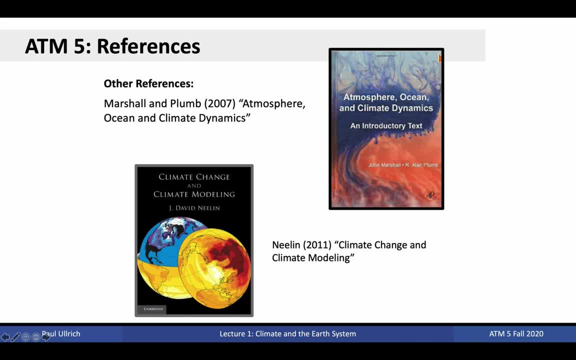 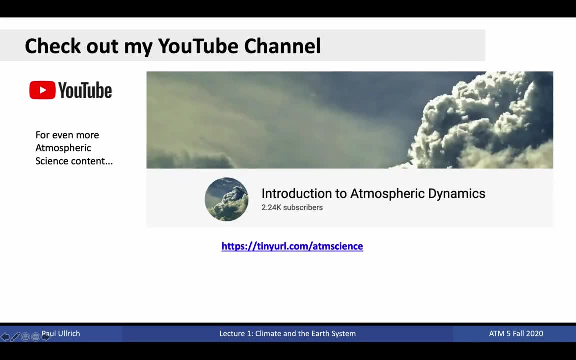 interested in learning more beyond what we teach in this class, in particular, about what techniques scientists use in order to understand the climate system. So if you're interested in learning more about climate dynamics, you can go ahead and check out my YouTube channel. Introduction to Atmospheric. 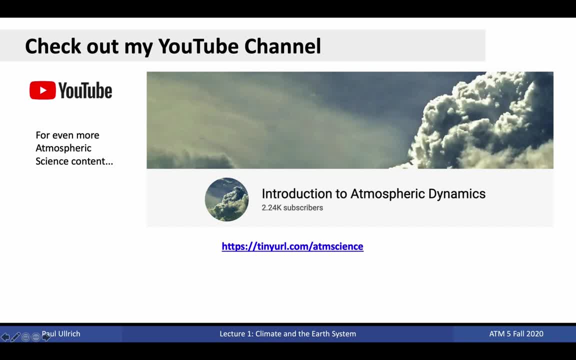 Dynamics, which you can find by just googling Introduction to Atmospheric Dynamics, or you can follow this tiny URL link shown here. The channel includes videos not only from this class, but also includes videos from when I taught atmospheric dynamics, which is ATM 121A and 121B. 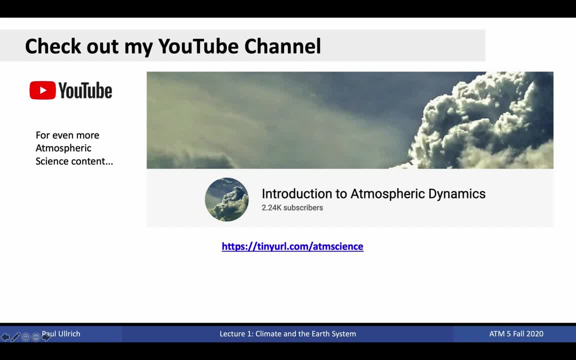 as well as climate dynamics, which is atmospheric dynamics, and atmospheric dynamics, which is atmospheric science. 241.. Feel free to check it out if you're interested in learning more about atmospheric science or just really like hearing me talk about things. All right, so I always like. 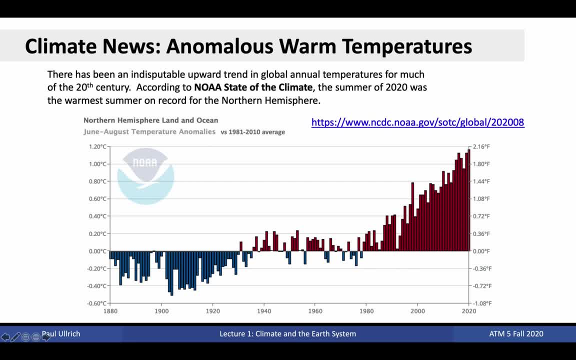 to kick off this course with a look at how climate change has shown up in the news. One of the primary references to track the science of climate change is actually the NOAA State of the Climate Report, which comes out every month. The most recent report that I'm working from here is the September. 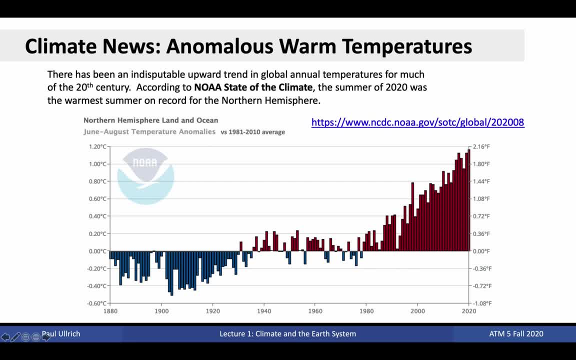 Report which covers material all the way through the end of the year. So if you're interested in learning more about climate change, you can check it out at the end of August, Since NOAA has access to a wide array of different observing stations and a copious data set of past climate data. 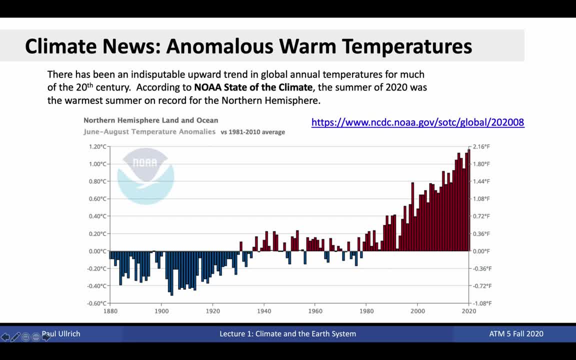 it provides an expert look at how the global climate system has been changing In 2020, it's well. it's been an interesting year, to say the least. We've suffered pandemics, politics and extreme weather. As climate change continues to intensify, we are also 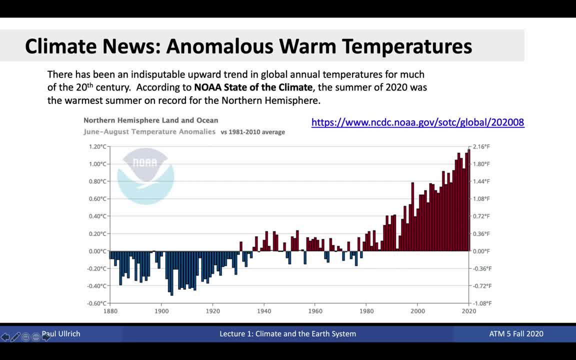 continuing to experience anomalously warm weather all over the globe. This is a natural consequence of climate change, and one that we'll be studying in detail over the next few weeks. Every month, basically for the past several years, we seem to be experiencing some sort of new record being. 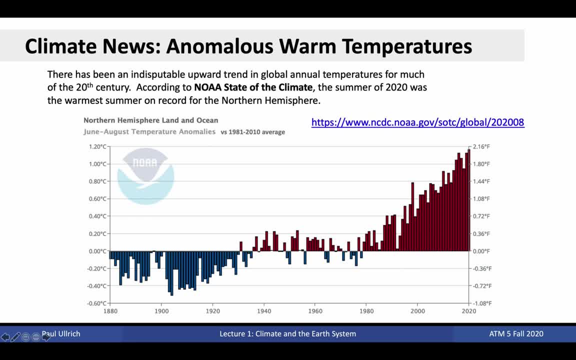 broken. Looking back over the summer of 2020 in particular, NOAA reports that the Northern Hemisphere has actually experienced the warmest summer on record, And actually here in California we've experienced the warmest summer on record, And so we're going to look at some of the 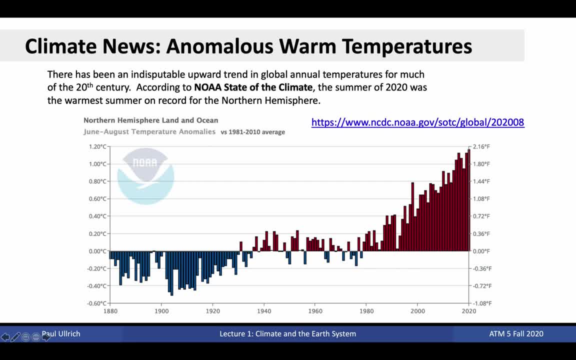 temperatures that we've experienced the warmest August on record. If we look closely at this graph, we can actually see that the last six years have also been the warmest six years on record for the Northern Hemisphere, And this is no coincidence. Just to get that out of the way this can be. 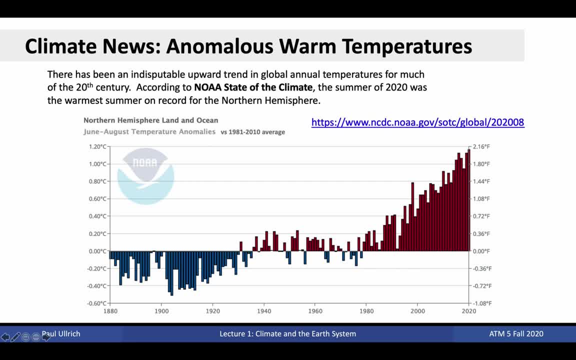 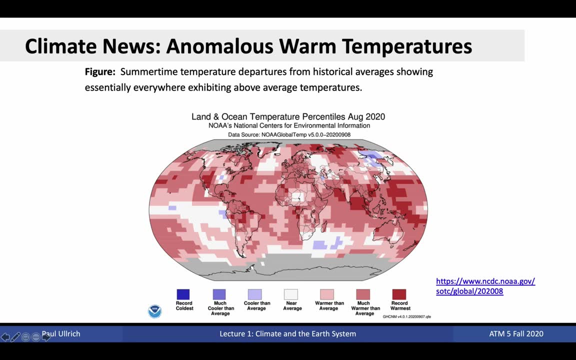 directly attributed to human activity and human emission of greenhouse gases to the atmosphere, which causes near-surface warming and consequently anomalously high temperatures. North America has also experienced its warmest August on record, at about 1.52 degrees Celsius, or 2.74 degrees Fahrenheit above average, And globally this was the third warmest summer on record. 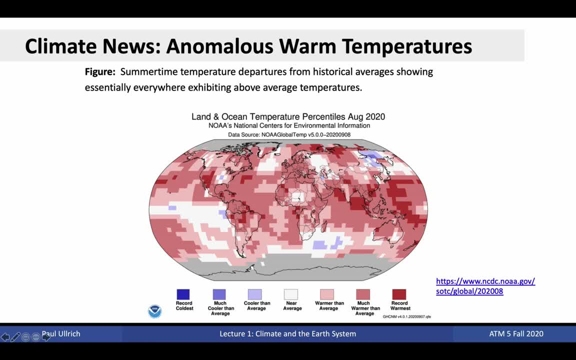 a record currently held by 2016,, which was an anomalously strong El Nino year. Later in the class, we'll talk about how instances of climate variability such as the El Nino event also influence these temperature records, as well as the global temperature. climatology Summertime. 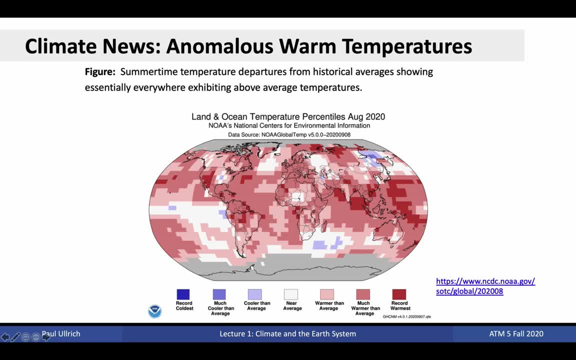 temperature departures from the history of climate change have also been a record, And so we're going to take a look at how these historical averages have showed up effectively- have basically showed that effectively everywhere on the globe is experiencing temperatures that are above average. Record warm conditions were observed in many places, including the Western. 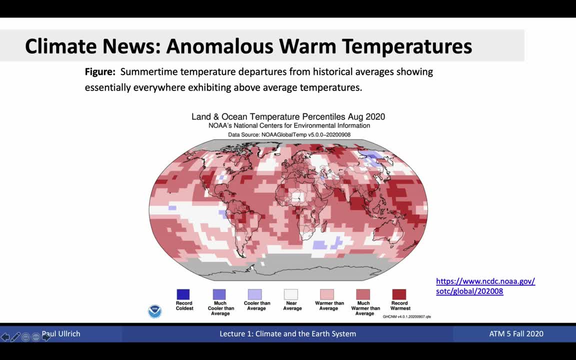 Equatorial Pacific, which you can see on the right-hand side of this particular map as well here in the southwestern US. As we'll learn from this class, these rising near-surface temperatures are a direct consequence of how we've been modifying the Earth's atmosphere, And this is 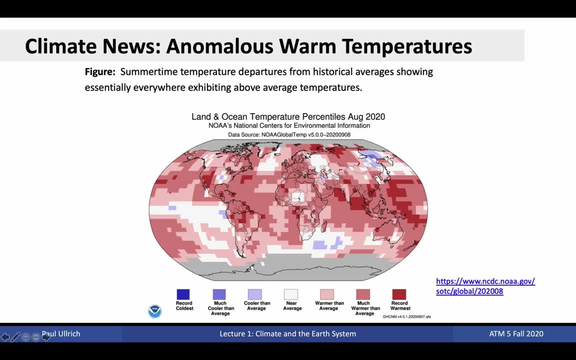 not particularly anomalous of what we should be experiencing in the years to come. Essentially, if we look at any month going forward, what we will see is continued records being broken of warmer and warmer temperatures On the extreme weather front. 2020 has also been a record-setting. 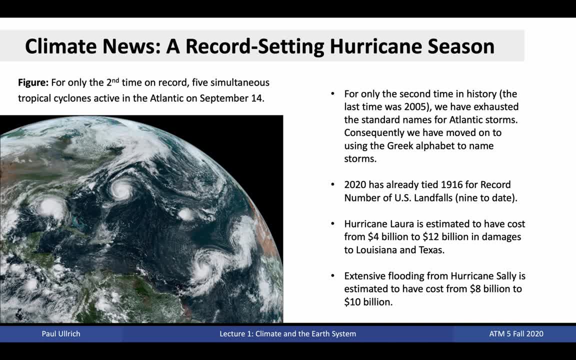 hurricane season- for those of you paying attention, And it's only September. The hurricane season will continue for the next couple months and likely result in even more records being broken. For only the second time on record, we've had five scientific studies show that the 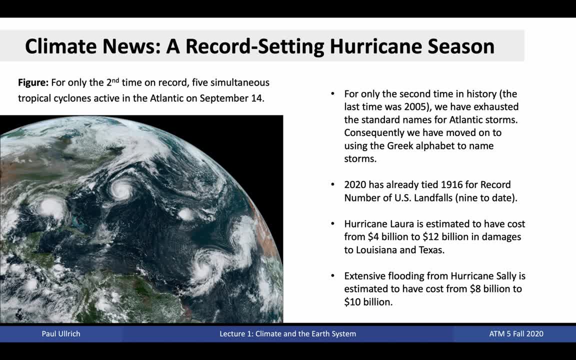 Earth has seen simultaneous tropical cyclones active in the Atlantic. This occurred on September 14th And for the second time in history. the last time was 2005,. we have actually exhausted the standard names for Atlantic storms. So far in the year, we've seen Hurricane Alpha, as well as Hurricane 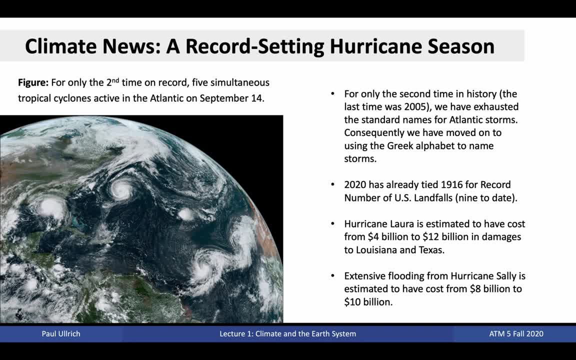 Beta show up in the Atlantic. We're going to continue using the Greek alphabet in order to name these storms and hopefully not exhaust the Greek alphabet as well. 2020 has already tied 1916 for a record number of US landfalls, And I think we're going to have to wait and see. 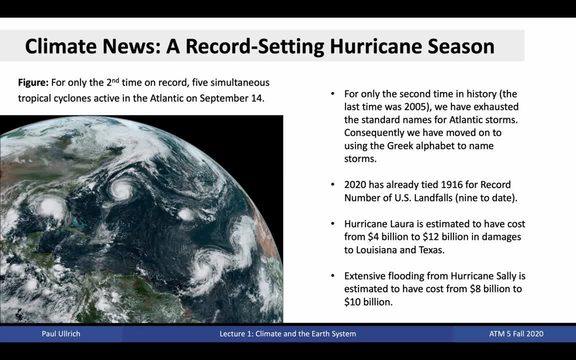 As I saw earlier today, there is only the west coast of Florida that has actually not been under a hurricane watch so far this year. The amount of damage associated with this hurricane season has been extensive and dramatic. Hurricane Laura is estimated to have cost from $4 billion to $12. 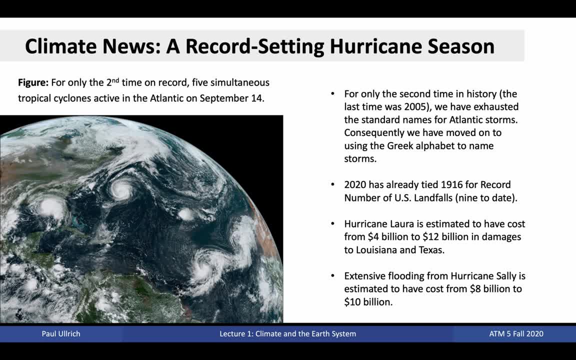 billion in total damages to Louisiana and Texas. Further extensive flooding that has been experienced from Hurricane Sally is estimated to have cost from $8 billion to $10 billion. As we'll learn later in the class, we'll be talking about how the hurricane has been. 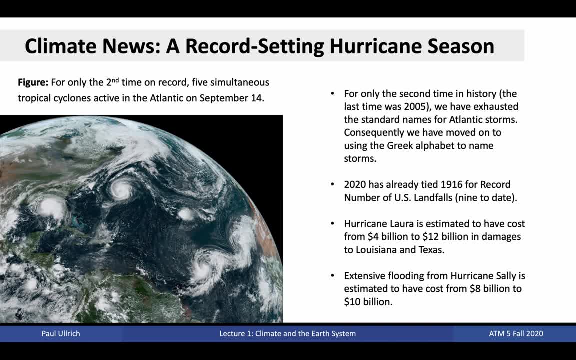 affected by climate change. Climate change has an indirect impact on tropical cyclones. Warmer ocean temperatures provide more fuel for these hurricanes, leading to more intense storms. Warmer air holds more moisture, leading to heavier precipitation and more extensive flooding. Sea-level rise caused by 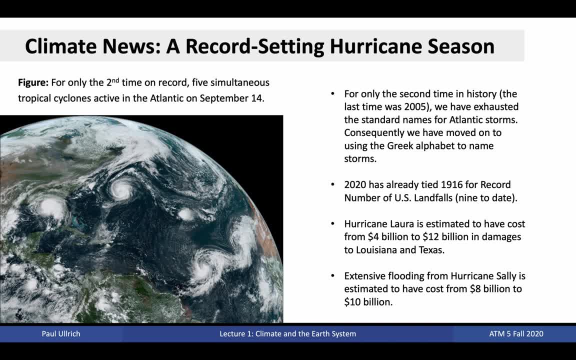 melting land ice and thermal expansion of the ocean waters is intensifying storm surge. However, contrary to what we've seen in 2020, our climate models also project a decrease in the total number of tropical storms, as more intense systems and major klipsch weather events are more disruptive to storms that follow in their wake. 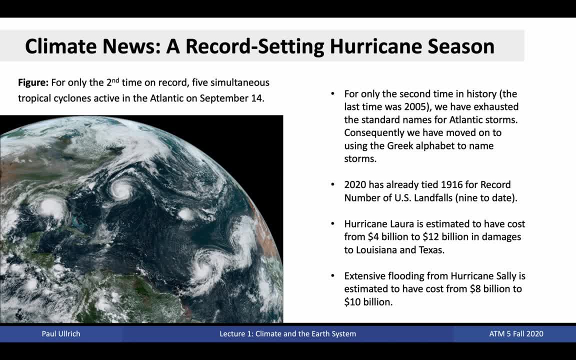 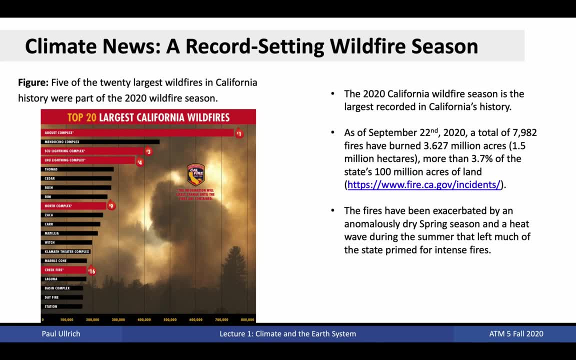 So, even though the tropical cyclone season tends to be highly variable, it seems that this year has been a particular anomaly, but that anomaly is still in the context of climate change. Here in California, we've also experienced a dramatic wildfire season. that is one of the 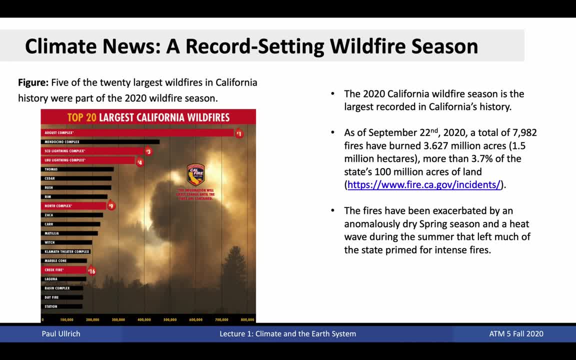 worst on record for modern civilization. Five of the 20 largest wildfires in California history were part of this 2020 wildfire season, And this is the largest recorded wildfire season in California's history. The effects again have been dramatic to us in the US West. 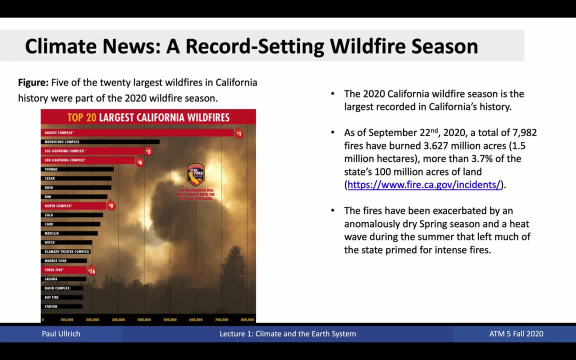 As of September 22, 2020, a total of 7,982 fires have burned about 3.6 million acres, or 1.5 million hectares, or more than 3.7% of California's approximately 100 million acres of land. 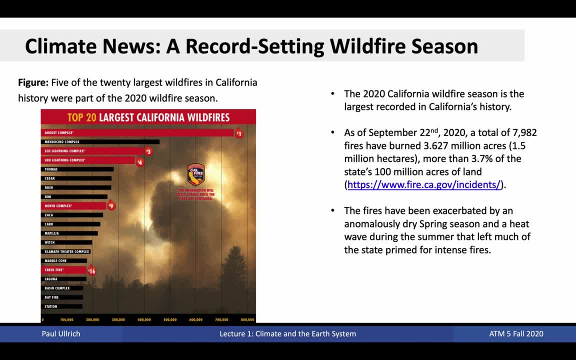 If you want to learn more about these fires, you can check it out on the CAL FIRE website link provided here. These fires have been exacerbated by an anomalously dry spring season and a heat wave during the summer that left most of the state primed for intense fires. 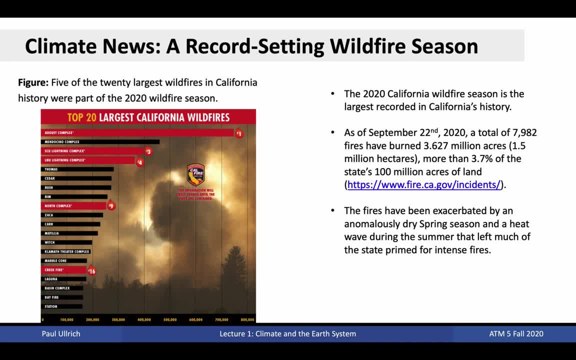 Studies have focused on how these fires are changing, and in the next lecture we'll talk a little bit about how wildfires are expected to change in response to climate change. Later in this class, we'll also be learning more about how climate change is causing the landscape of Northern California to transition. 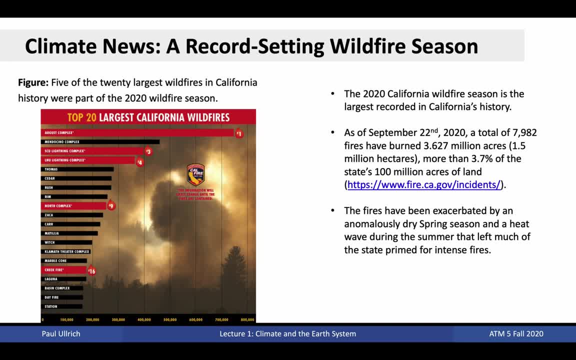 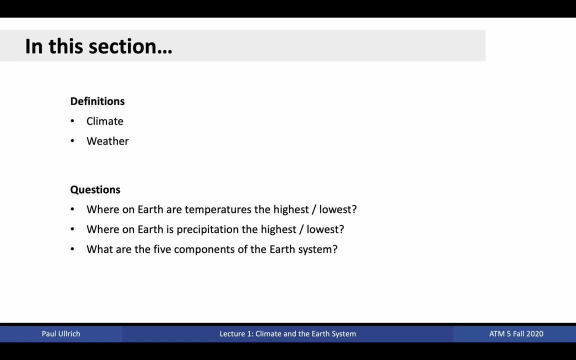 from the temperate forests to shrublands more constantly. While we Скip this part, let's also move on to the next fish, our останов in the theoretical field. This is a lot of information that we are searching for to prepare myself for my Bella conta Корan. 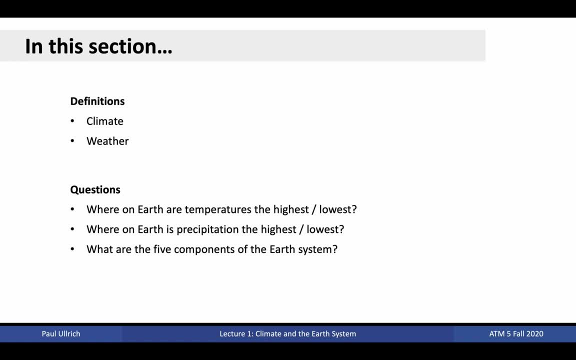 For this class. I'm a chemistry professor at the University of Obviously in the US and research senior scientist Rhodes Program calculator at the University of destrodich標. On this slide you can see a reflection of new ». In this last section we're going to learn some of the differences between principalmente wet and not wet time range. 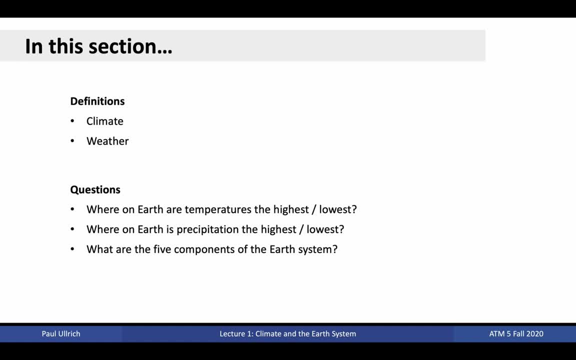 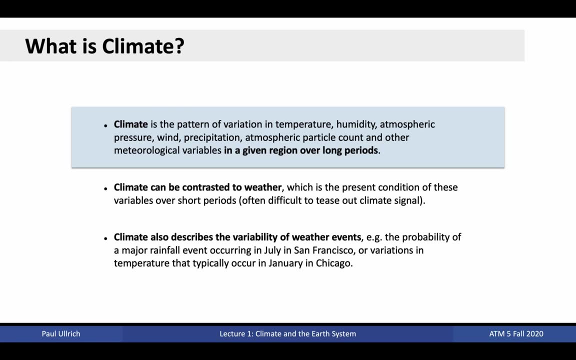 as well as weather- highest and lowest- And what are the five components of the Earth's system. Alright, let's get started by defining climate and contrasting it against weather. So climate is the pattern of variation in temperature, humidity, atmospheric pressure, wind precipitation. 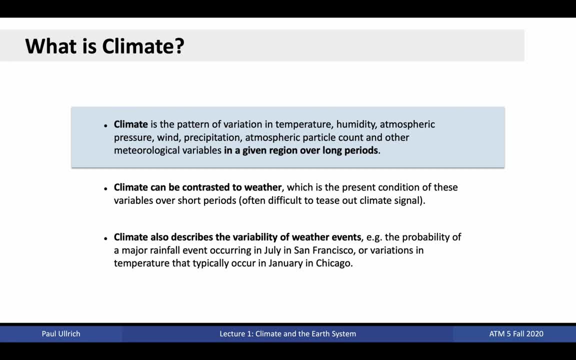 atmosphere, particle count and other meteorological variables in a given region over long periods. I emphasize that these last six words are particularly important for defining climate, That is, you have to define a location for which you're talking about the climate As well. 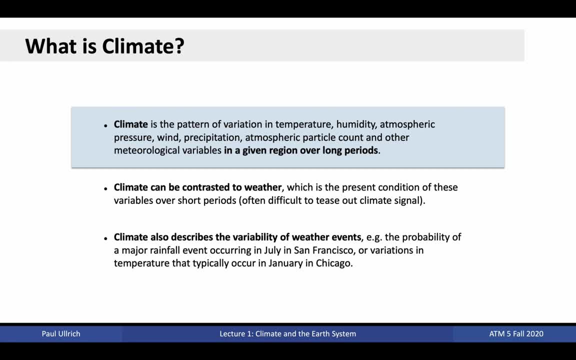 climate must occur over a long period of time. Here we're talking about the statistics of weather, not specific weather events. Thus climate can be contrasted to weather, which is the present condition of these variables over short periods. So this is different than the 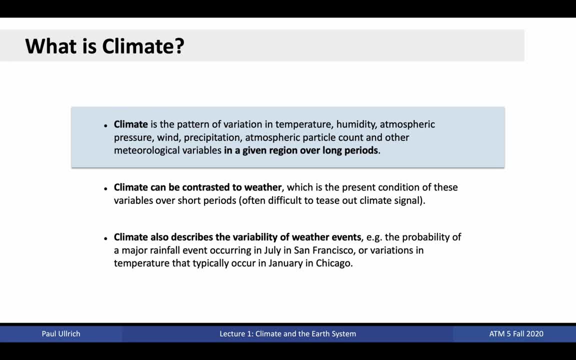 climate signal which is over a long period of time. Often, you have strong variation in things like temperature, humidity, atmospheric pressure, humidity, atmospheric pressure, humidity, daily temperatures. The daily temperatures themselves, though, are individual weather signals, but they exist on top of a long-term history of average conditions, known as the. 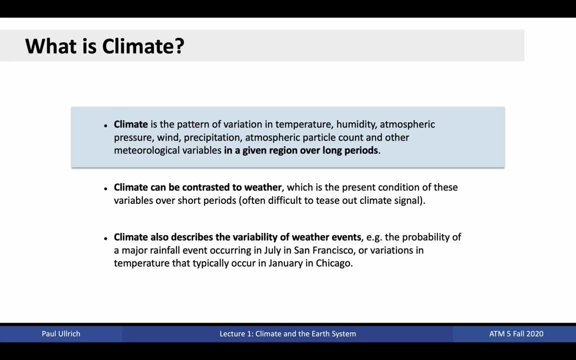 climate. As the climate warms on average, what we tend to see is more instances of warmer weather events as well, But again, those occur on this backdrop of the average climate. Climate also describes the variability of weather events, namely things like the probability of a major 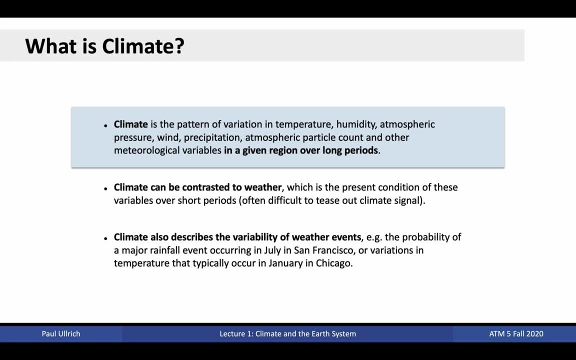 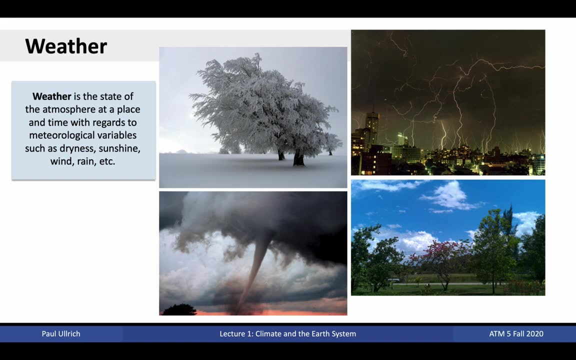 rainfall event occurring in July and the probability of a major rainfall event occurring in July. In some sense, you can again think of climate as the statistics of weather. Weather, on the other hand, is the state of the atmosphere at a place and time with regards to 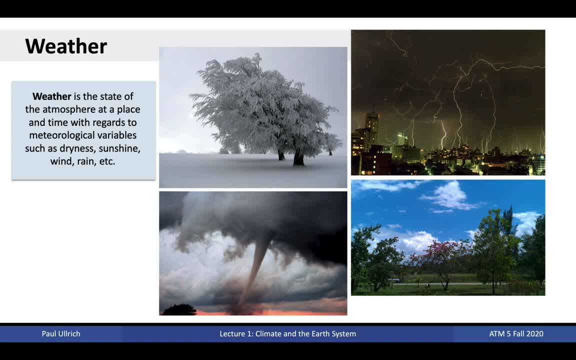 these meteorological variables. So if a snowfall occurs, that's a weather event. If a tornado occurs, that's a weather event. If you have a lightning storm, that is a weather event. That is a short time scale event that affects a particular location. So if you have a storm, 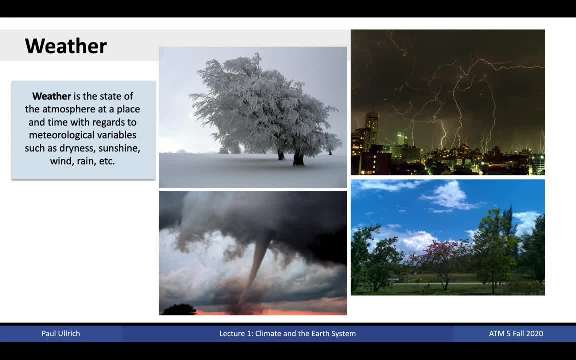 that's a weather event. So if you have a lightning storm, that's a weather event. So if you have a location or region, Nice weather also is a weather event. That is, it's the state and conditions of the meteorological variables at a particular point in time. When you average all those weather events, 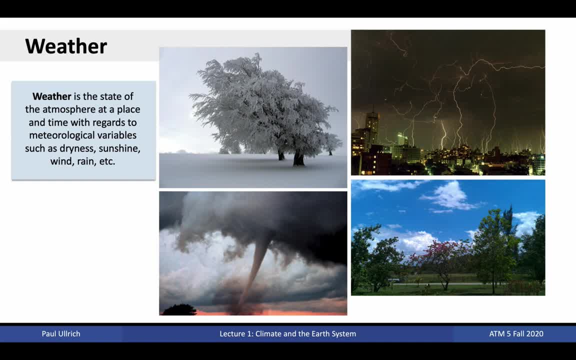 over time. that gives you the climatology of the region. Things like the probability of a snowfall or the probability of a tornado or the probability of nice weather are all climatological variables. There's a nice way in order to construct this idea. 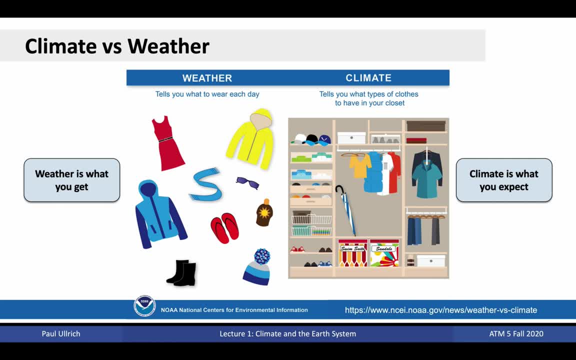 Climate versus weather. Weather is basically what you get. It's what you're wearing today. What you're wearing today is in response to the weather of the day. Climate, on the other hand, is what you have in your closet. You have all sorts of clothes in your closet to prepare you. 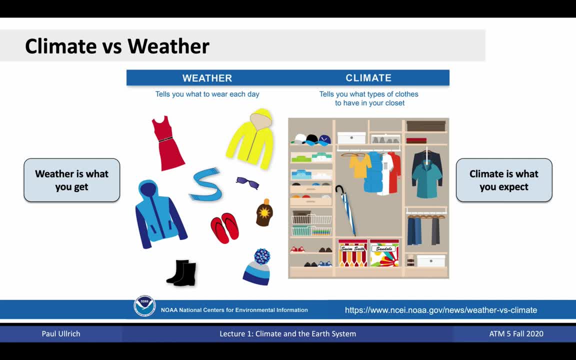 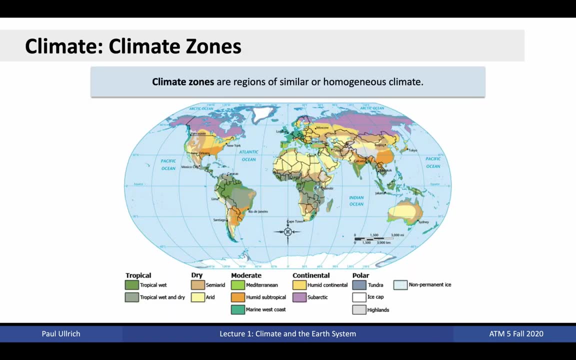 for the types of weather events that could occur on each day where you live. Consequently, you have a large statistical sample, many different days of weather, all stored within your climate closet. In order to understand what people have in their various closets worldwide, we typically break the 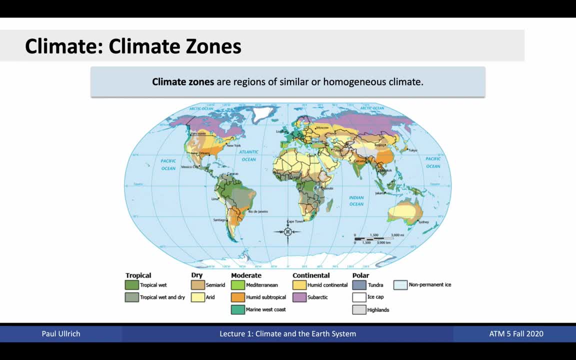 world up into what are known as climate zones. These climate zones are regions that of relatively similar or homogeneous climate. It's common to classify these zones by what is known as a Copen climate classification, such as the one shown here. The climate of the world is affected. 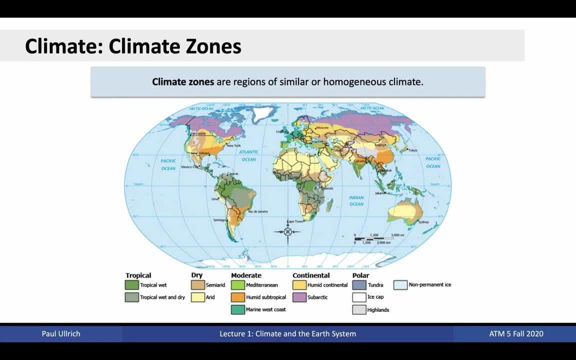 primarily by temperature and precipitation. Polar regions are cold. Equatorial regions are cold. Precipitation is generally higher at the equator and varies depending on the location. elsewhere, Depending on that combination of temperature and precipitation, we can divide the world up into. 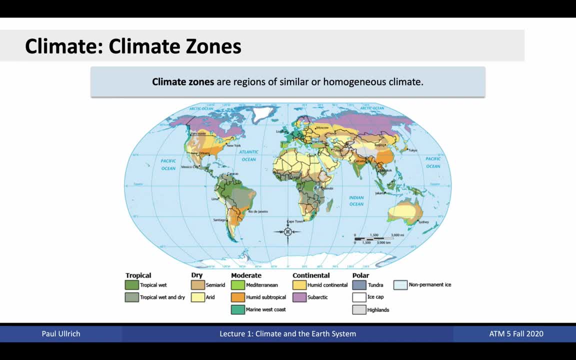 tropical, dry, moderate, continental and polar climate zones, and then subdivide those further based on the average climatology in each of those regions. In order to understand what gives rise to these climate zones, we must then study the temperature and precipitation of the world. 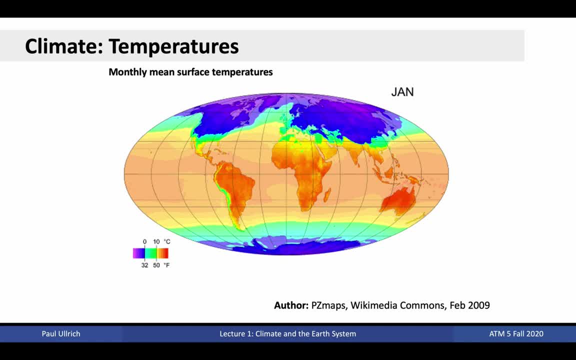 As mentioned before, temperature has a pretty basic variation over the Earth's surface. The warmest temperatures are found near the equator or the middle of this plot. The coolest temperatures are found towards the poles or the top and bottom of this plot. Also, as you tend to go to higher, 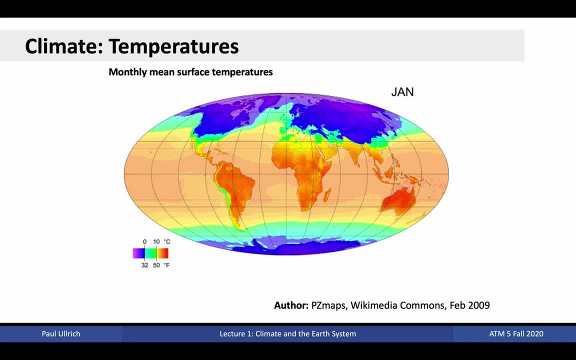 elevations, you also tend to find cooler temperatures. overall Temperature also varies throughout the year depending on where the Earth is in its orbit. In December and January, the tilt of the Earth causes the southern hemisphere to be facing more directly at the sun. consequently, 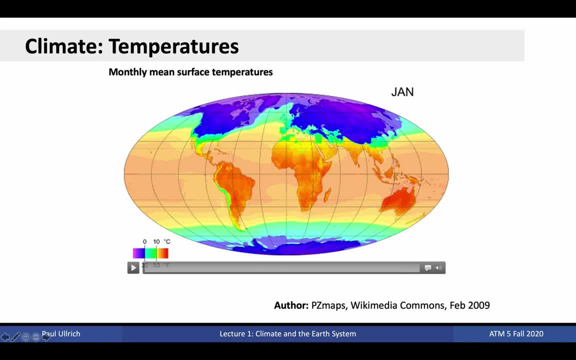 driving the Earth to the south. In the summer the temperature of the Earth is higher and the temperatures in the southern hemisphere are rising As we move forward in the year. we have the sun now moving from overhead in the southern hemisphere to being overhead in the northern. 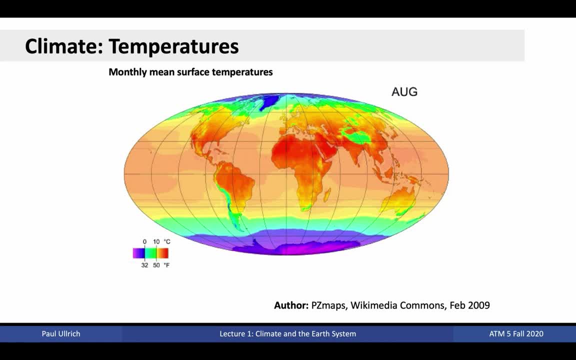 hemisphere. Consequently, this region of maximum temperatures also moves with the sun. During this season we see warmer temperatures in the northern hemisphere and cooler temperatures in the southern hemisphere In particular. you see here, Antarctica becomes very cold in this northern hemisphere summer season. 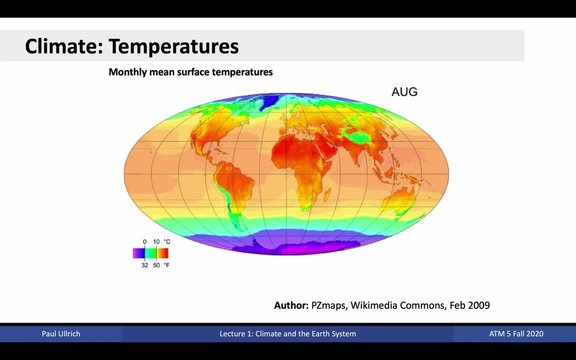 Temperatures are generally warmest around the equator, although that point of maximum temperature does tend to follow the sun. north and south Temperatures are also affected by differences between ocean and land. It takes much more energy to warm up ocean water than it does to warm up land. 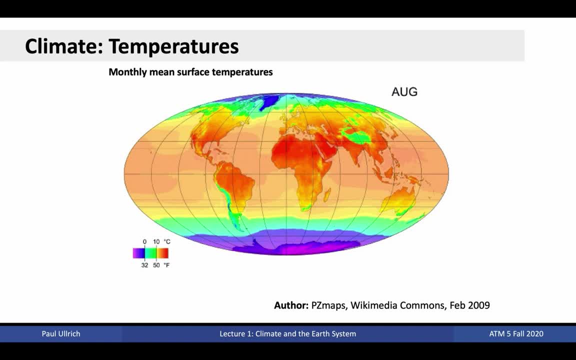 It's also much easier for the land surface to lose its energy through radiation and evaporation. As a consequence, ocean temperatures tend to be much more stable than over land, where we see much more dramatic shifts in temperature between seasons. This is also one of the reasons why coastal regions typically tend to be much more mild. 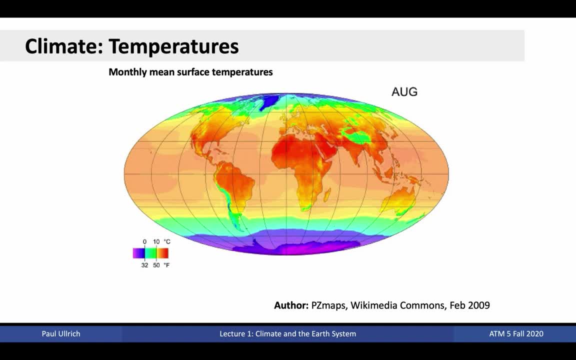 and have a weaker temperature variation than more inland regions. The ocean is a natural regulator of temperatures and thus provides those coastal regions with modulation of their temperatures. Finally, temperatures are also affected by dynamical patterns of the earth's system: The gulf stream, which goes from the Gulf of Mexico northeast through the Atlantic Ocean. 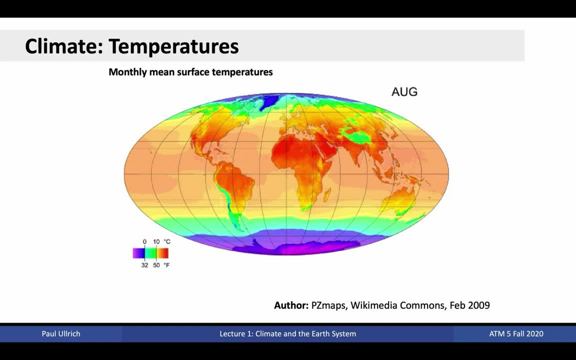 is responsible for transporting warm water to promote a shallowushi level across the Atlantic. It's also responsible for pushing up temperatures in Europe. Because of this pattern, we see warmer waters in Europe at the same latitudes that we see them in North America. Wintertime temperatures in Goose Bay, Newfoundland. 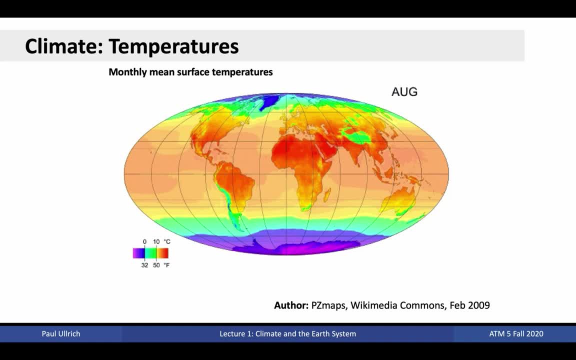 are around minus 18 degrees Celsius. In Dublin Ireland, which is at approximately the same latitude, wintertime temperatures are rarely below freezing. That's about here for Goose Bay, about here for Dublin Ireland In general. because of these weather and oceanic patterns. 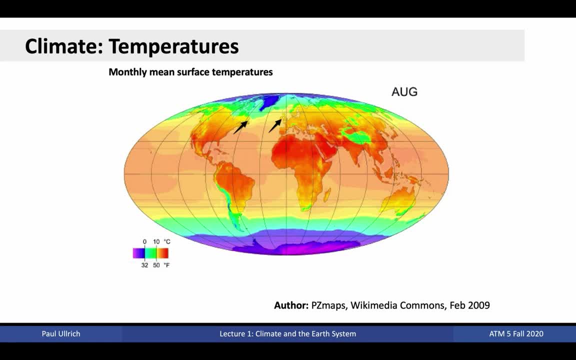 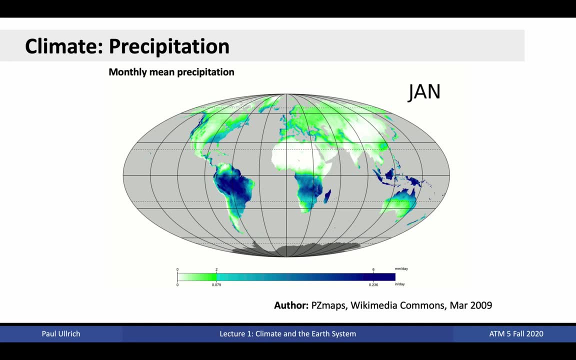 the west coast of these continents tends to be significantly warmer than their east coasts. Looking at precipitation, we see that the wettest regions of the world are around the equator. This is because of convergence and lifting of moist air in a region known as. 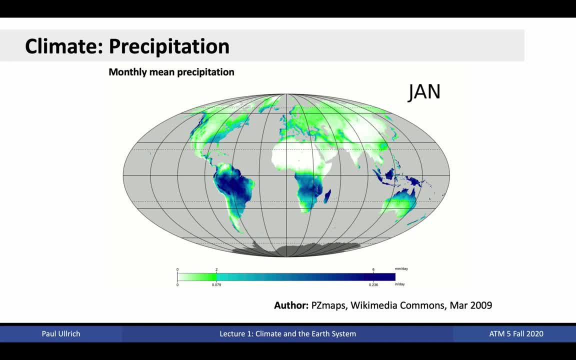 the Intertropical Convergence Zone, or simply the ITCZ. This is also where we'll find most of the rainforests of the world. This wet band tends to follow the sun north and south with the seasons as well, as we will see As the sun moves into the northern hemisphere. 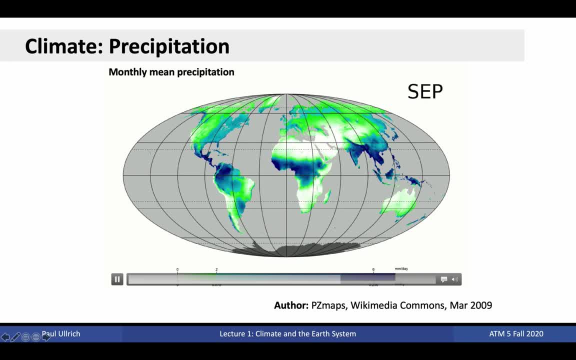 that region of intense precipitation moves along with it, And as the sun moves back to the southern hemisphere, in December we have that the wetter regions also move to the southern hemisphere. To the north and south of the ITCZ are the subtropical convergences. 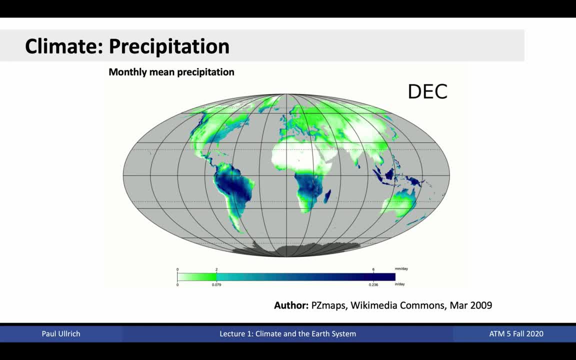 latitudes where descending air from the ITCZ naturally suppresses precipitation and drives drier conditions. This is also where we'll find the deserts of the world, including the Sahara in the Northern Hemisphere, as well as the Kalahari and the Great Australian Desert in the south, Going again poleward, we 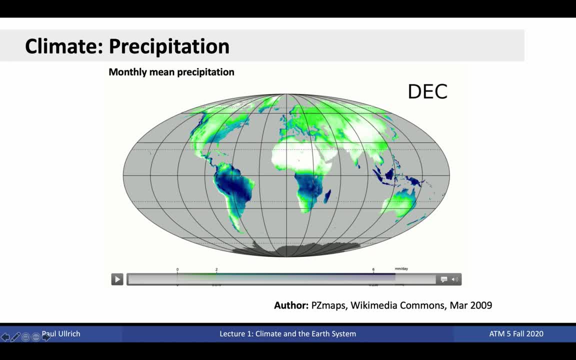 enter the mid-latitudinal regions. here In the mid-latitudes there's strong longitudinal variation in precipitation amounts. As you can see, along the western coast of the United States this is typically very wet in the winter season. Then we have drier conditions through the mountains as well as more modulated. 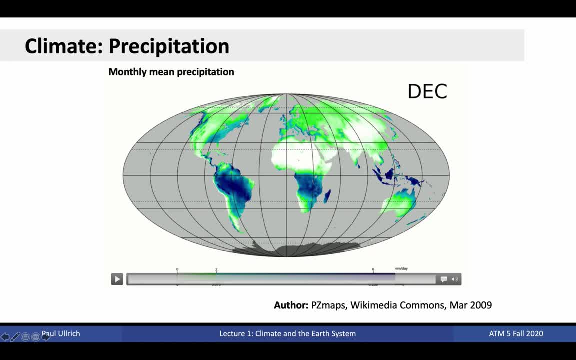 conditions in the eastern US. Similarly in Europe and Asia. we see wetter conditions along the western coast of Europe and drier conditions as you go farther inland. in Asia, California, as we know, is very wet in the wintertime and dry in the summertime. The east coast of the US, on the other hand, where? 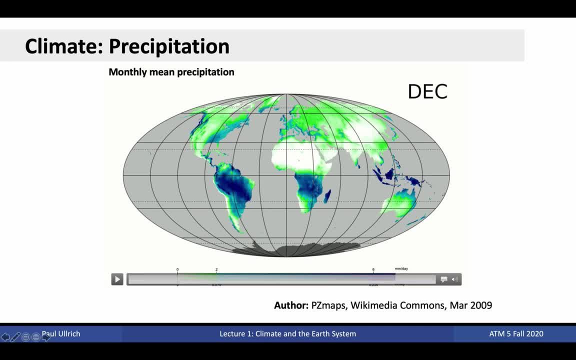 precipitation mainly comes in the form of transport from the Gulf of Mexico over land tends to have a relatively same amount of precipitation regardless of what time of year it is. If we go farther north still, we enter the polar regions, and this is where we again find incredibly dry conditions, because the cold air of these regions cannot. 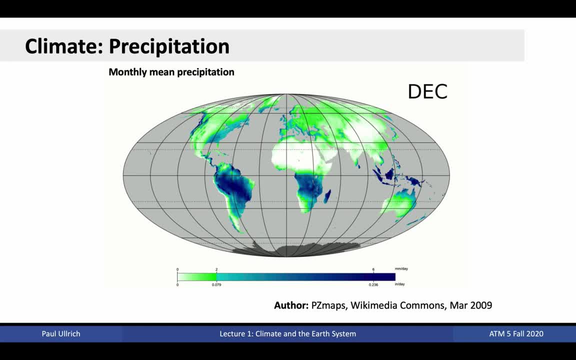 hold on to atmospheric moisture and, consequently, that moisture cannot be used to generate precipitation. The driest regions of the world can actually be found in these polar regions, With the driest region of the world actually found in what is known as the dry valleys of 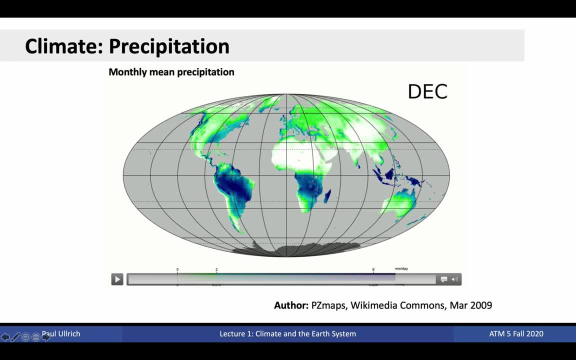 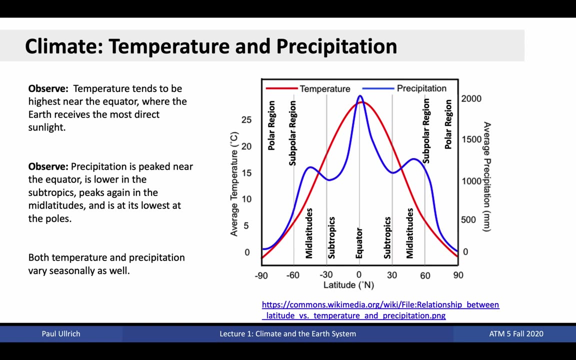 Antarctica, where the average precipitation is essentially 0.. Even for the large deserts of the world, it's very rare to find locations where you have absolutely zero precipitation. Combining these two plots and averaging across longitudes, we obtained the chart shown here, where you have the southern 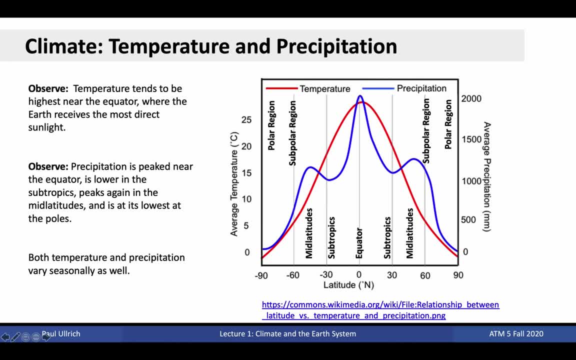 hemisphere on the left of the plot and the northern hemisphere on the right of the plot. The red line shows the temperature variation. This plot shows the qualypsoic radiation 大셨 acquainted The力ommes and тел battery change pakai. 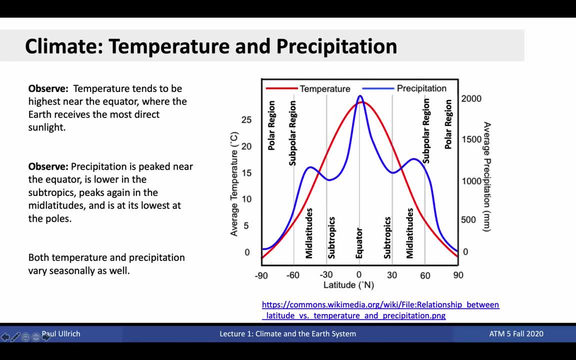 The red line shows the temperature variation. This plot shows the as a function of latitude and the blue line shows precipitation variation as a function of latitude. As in the previous discussion, we've broken up the Earth by latitude into a variety of regions, including the equatorial zone, the subtropics, the mid-latitudes, the subpolar region. 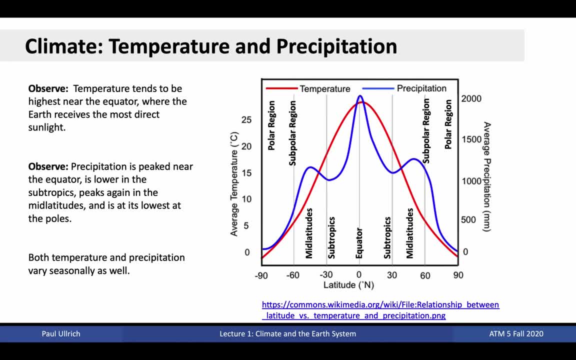 and the polar region. Average temperatures globally vary between 27 degrees Celsius at the equator and negative one degree Celsius at the poles. Average precipitation varies from 2,000 millimeters per year near the equator to approximately zero near the poles. Obviously, 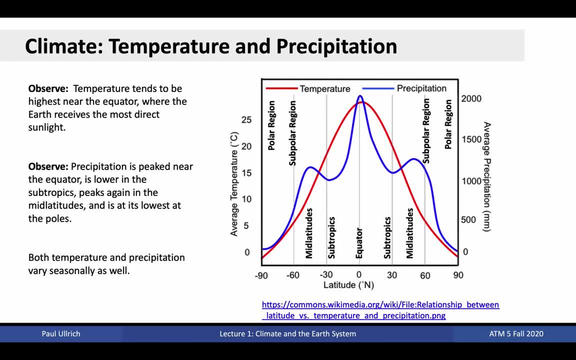 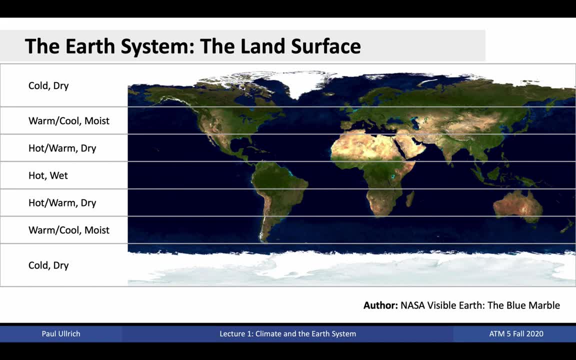 these two variations then have the potential to create very diverse climate zones across the planet. Breaking up the Earth's surface into zones based on temperature and precipitation, we see that the equatorial bands tends to be hot and wet, the subtropics tend to be hot, slash warm. 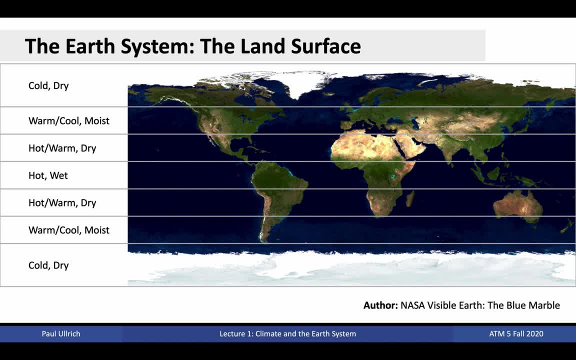 and dry, and the mid-latitudes vary between warm and cold, But remain relatively moist depending on where you are on the continent, And the subpolar and polar regions are cold and dry. We can see what effect this has on the Earth's land surface, shown here in a NASA visible Earth image where clouds have been digitally. 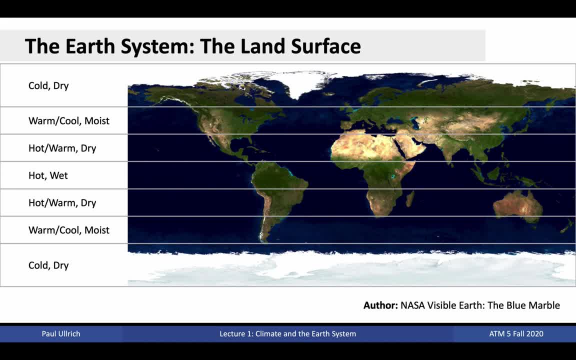 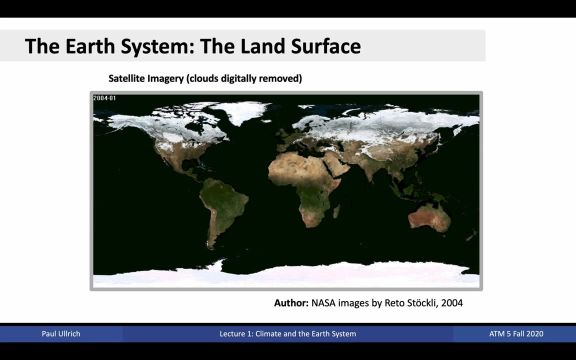 removed. Greener regions correspond to vegetation requiring nominal levels of precipitation and warmth. Brown regions are the deserts of the world, generally found in the subtropics. White regions are covered in snow and ice. Of course, the land's surface varies throughout the year as seasons change. At the beginning of 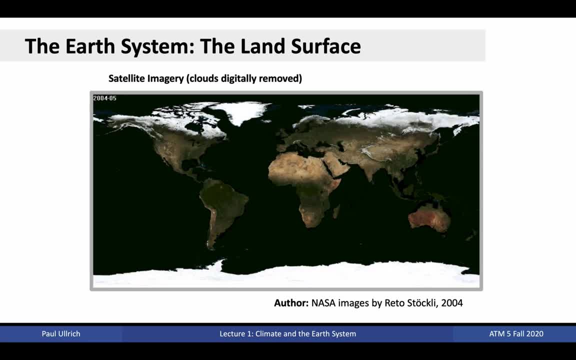 this animation we see a cold and snowy northern hemisphere. in January, The sun is in the southern hemisphere, and so precipitation is enhanced. south of the equator, As we move throughout the season, the snows retreat and precipitation shifts northward. The edges of the deserts move with. 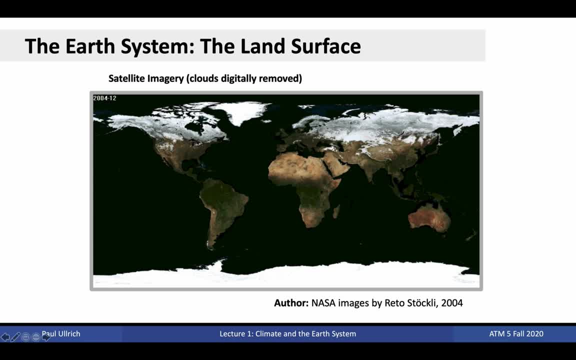 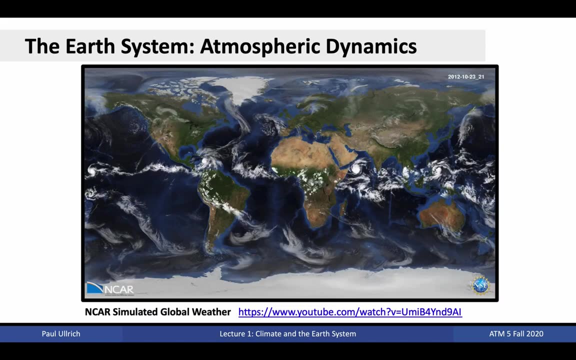 the rains In the northern hemisphere. summer, the Sahel region of Africa experiences the African monsoon, leading to its greening. Simultaneously, California becomes dry as the desert region edges move to the north. These shifts in the land surface are occurring within the context of a highly chaotic atmosphere. 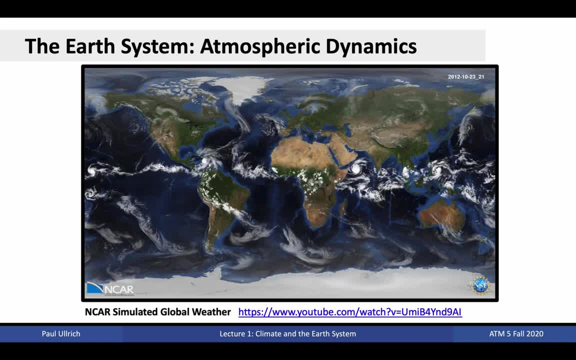 In this snapshot from a simulation of global weather patterns, we see sharp and spotty cloud patterns across the equator in the ITCZ, associated with deep convection. Here, air is being violently drawn upward from the surface of the equator. In this snapshot, we see sharp and spotty cloud patterns across the equator in the ITCZ, associated with deep convection. 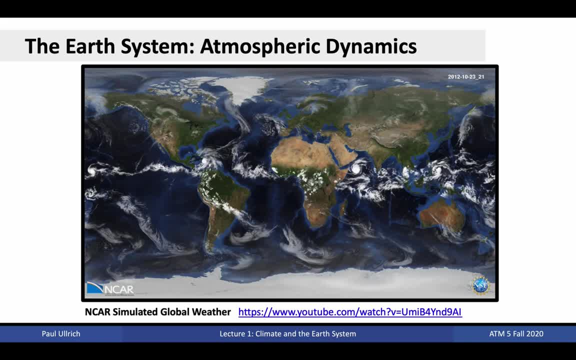 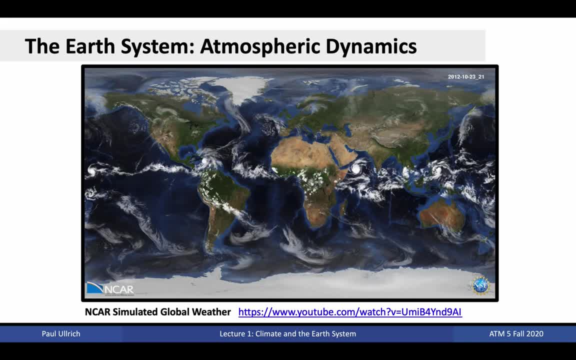 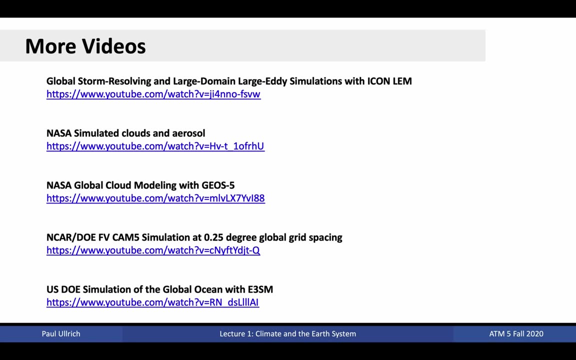 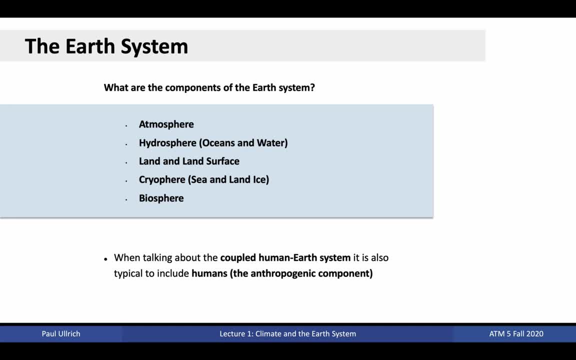 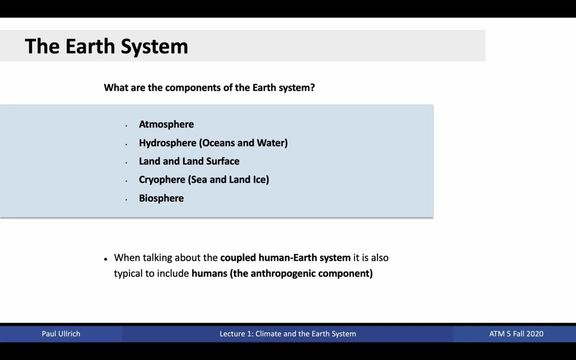 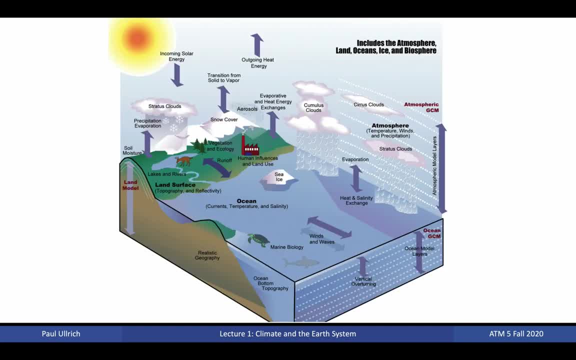 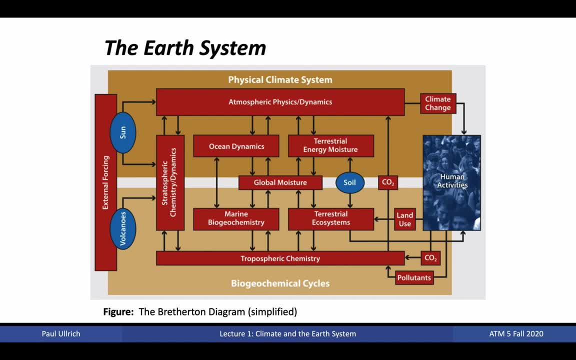 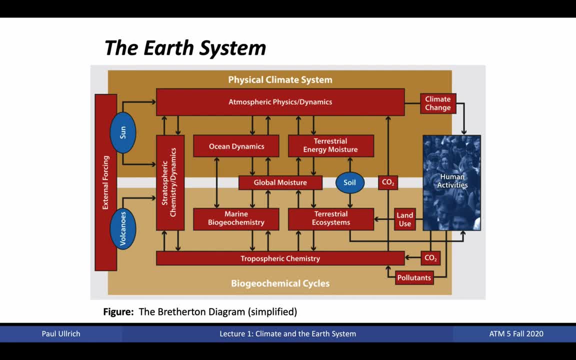 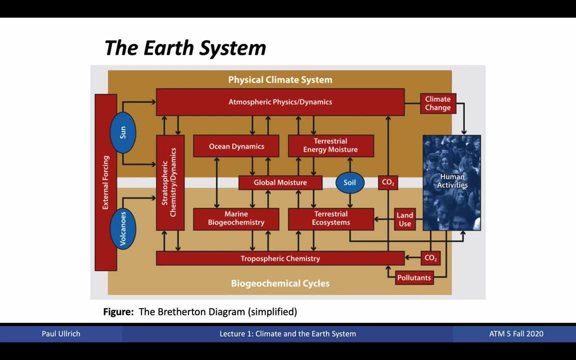 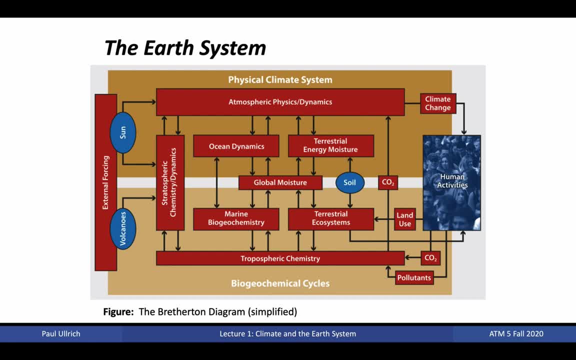 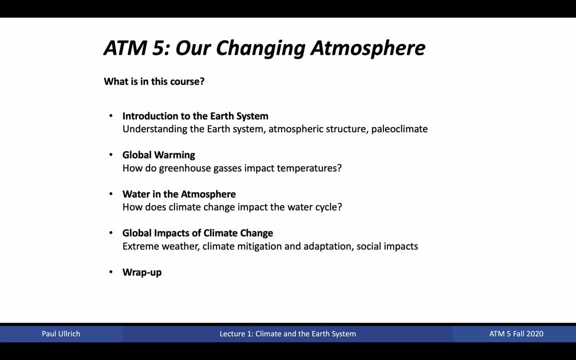 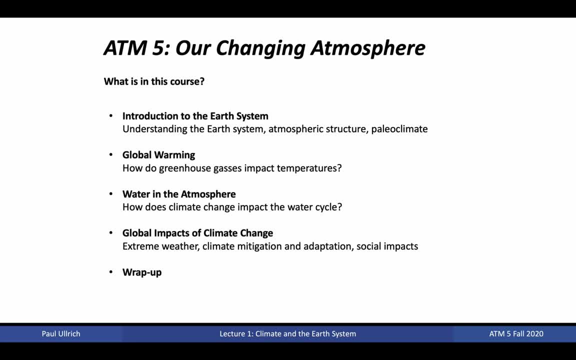 atmosphere. We're going to then talk about global warming and answer the question: how do greenhouse gases impact temperatures? Then we're going to talk about water in the atmosphere. Water is inevitably a major component of the cycles of the Earth's system, So we're going to ask: how does